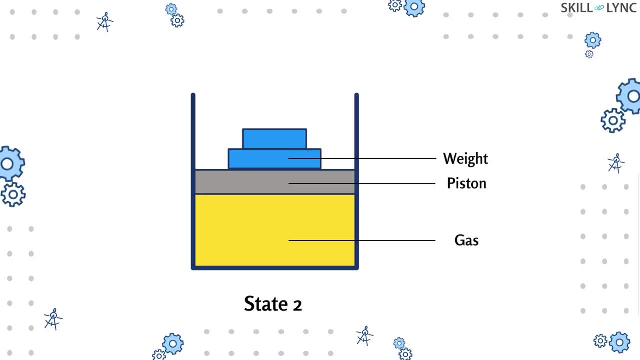 the system changes. Let's call this new state as state 2.. Similarly, another weight is removed and the new state- let's say state 3, is obtained. Finally, the last weight is removed and the final state is obtained. We'll plot this on a p-v diagram. As you can see, there are two intermediate. 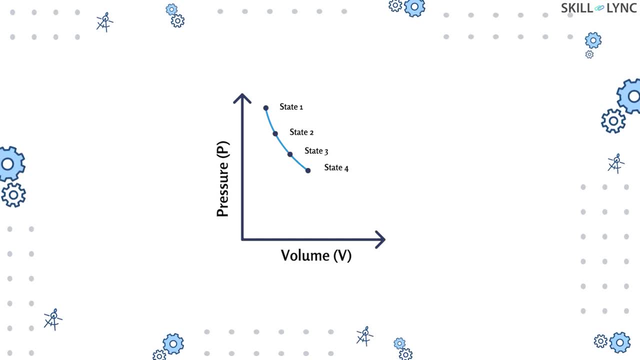 states between state 1 and state 4, namely state 2 and state 3.. This means that the gas under compression has to pass through states 2 and 3 to reach state 4.. According to the theory of quasi-static process, this change in state is infinitesimally slow And it can be assumed that 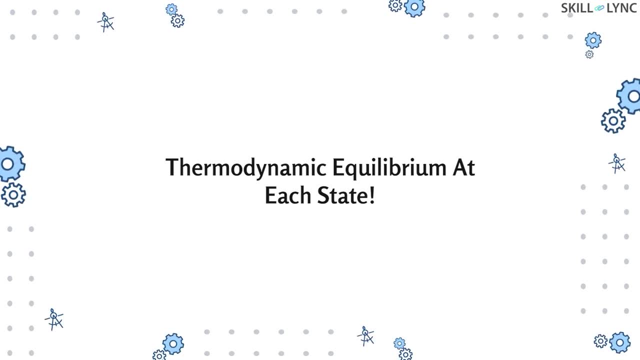 a thermodynamic equilibrium is established in each of the intermediate states. In simpler terms, a quasi-static process is an ideal process in which a change of state occurs at an infinitesimally slow speed, such that a thermodynamic equilibrium is established in the system at 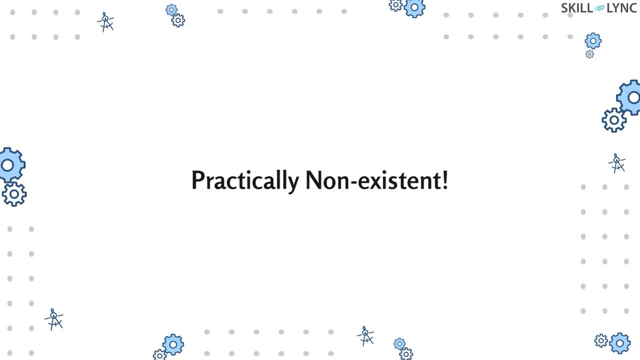 each instant. Such a process cannot be completely realized and hence all processes going on in nature are non-quasi-static. Now let's move on to discuss what is reversible and irreversible process. In thermodynamics, a process is said to be reversible if it can be reverted such that 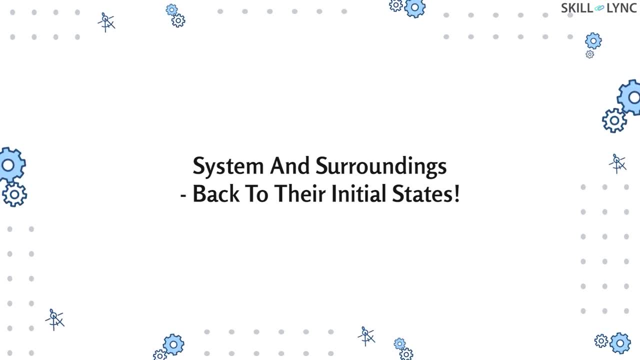 system and surroundings get back to their initial states. There should be no other change anywhere else in the universe. In reality, completely reversible processes do not exist. Even in the example of melting ice that we talked about earlier, there is always a small part, which 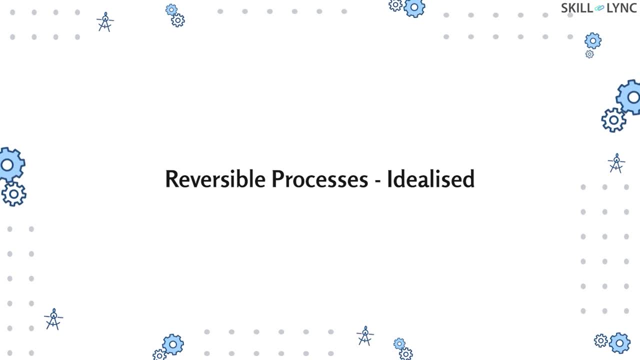 cannot be completely turned back. The reversible processes are idealized cases of real processes. The purpose of creating these idealized cases is to determine the maximum efficiency a system can provide. A few examples of such reversible processes are: extension of springs, slow, adiabatic. 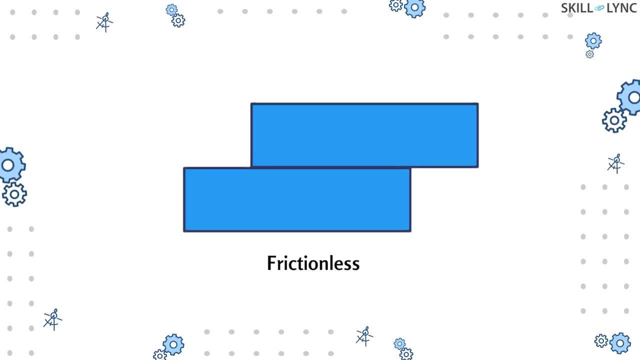 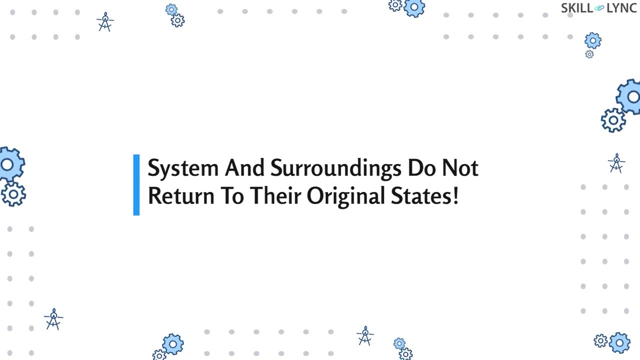 compression or expansion of gases and frictionless motion of solids. On the other hand, there are thermodynamic processes in which the system and surroundings do not revert back to their initial states. Such processes are called irreversible processes. You can consider the burning of fuels as an example for this. When we operate a vehicle using fuel, the combustion